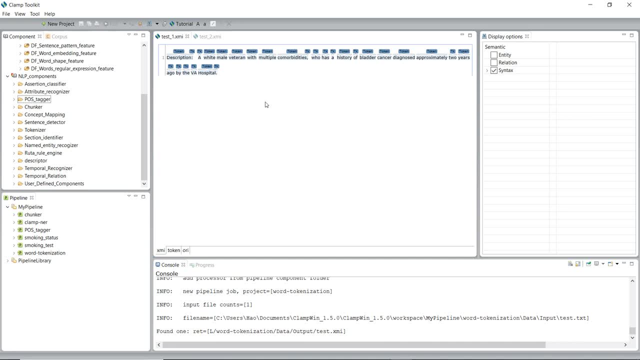 POS tagging is more complicated than just having a list of words and their parts of speech, because some words can represent more than one part of speech at different times. In natural languages, a large percentage of the word forms are ambiguous. Therefore, a POS tagging algorithm needs to look at both the word's definition and its context in the sentence. 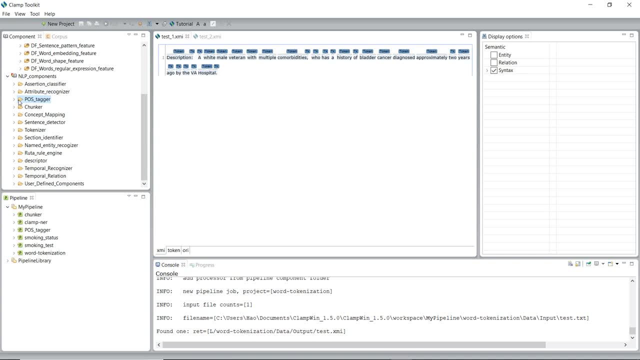 The CLAMP toolkit currently provides only one POS tagger, the default OpenNLP POS tagger. This tagger had been retrained on a dataset of clinical notes. Therefore it is designed specifically for clinical text. But for advanced users you can certainly replace the default POSbin model to your own model. 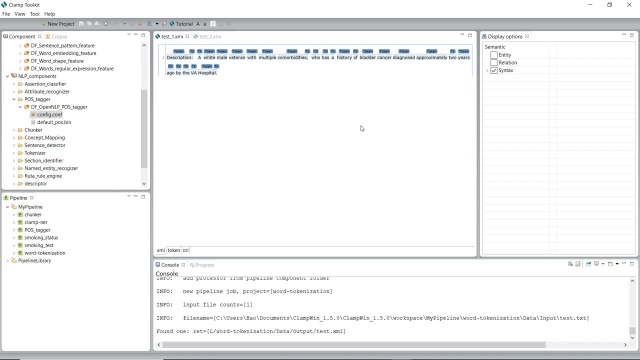 In the CLAMP toolkit. the part-of-speech information can be easily visualized when we hover our mouse over the tokens, such as comorbidity, For example. if a person uses one of these three words, one word will indicate the correct enamuttering term. 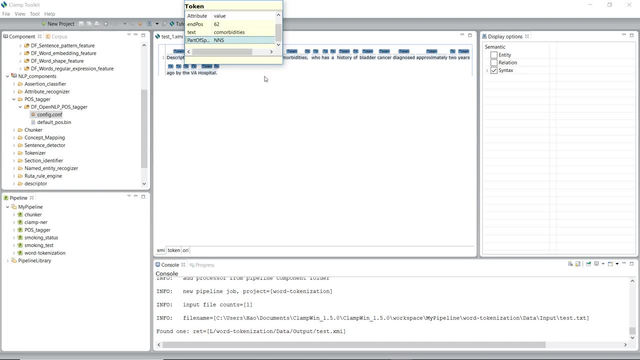 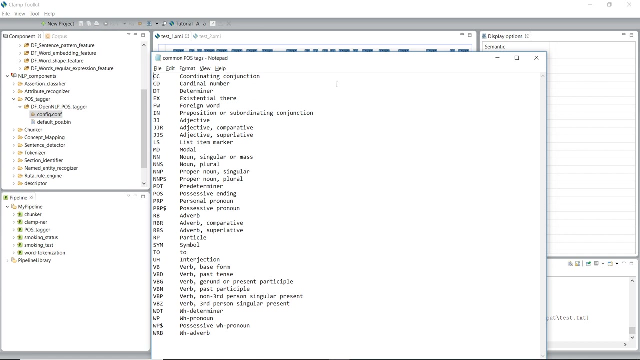 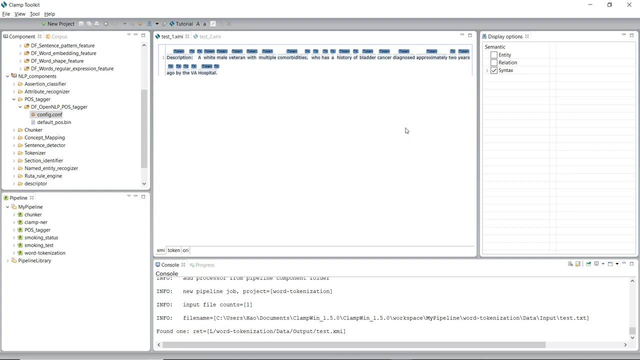 Such as word u Tick Angle Style. POS tags such as nn means noun, rb means adverb, vb means verb, just to name a few. Now let's talk about chunking. A chunker does a shallow parsing of a sentence and identifies. 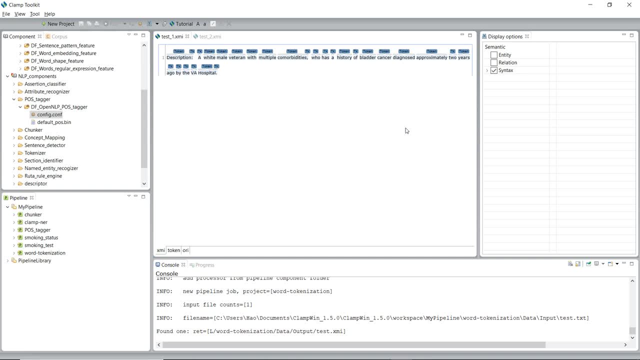 the syntactic constituents, such as noun phrases, verb phrases, etc. The process is similar to how we understand a sentence or memorize a telephone number. We don't try to understand a sentence by individual words or try to remember a phone number by individual numbers Instead. 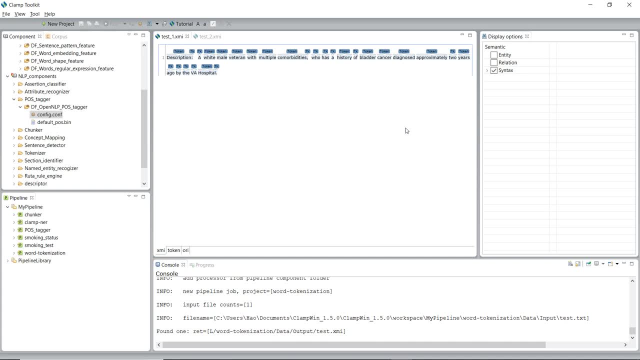 we group them together to make things easier to understand or remember. This is chunking, to chunk together information. In the CLAMP toolkit there is one chunker provided, the default openNLP chunker, which is a wrapper of the chunker in OpenNLP Again, advanced users.